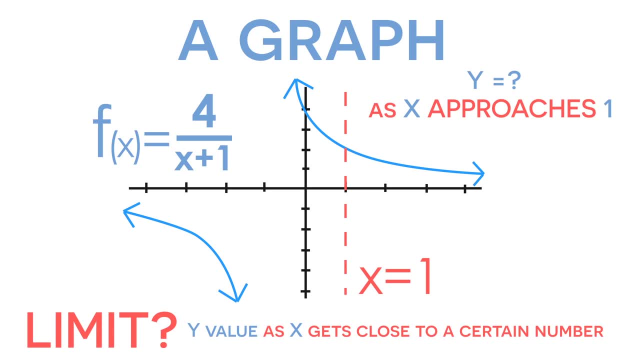 So let's do this right now. Let's see what the y value is going to be as x approaches 1, or x gets really close to the value 1.. And we have to approach x equals 1 from the right side and from the left side. 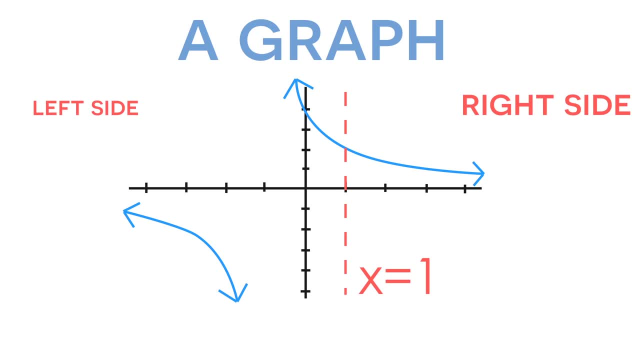 So let's start from the right side of x equals 1.. So if we put our pencil on the right side of this graph and we draw arrows going from right to left towards the line x equals 1, notice how the closer and closer we get to. 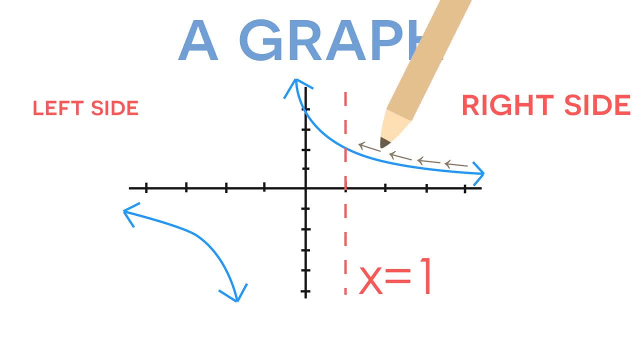 the line x equals 1, or as x approaches 1, the y value gets closer and closer to 2.. It gets infinitely close to the value of 2.. So as x approaches 1 from the right side, our y is going to be 2.. 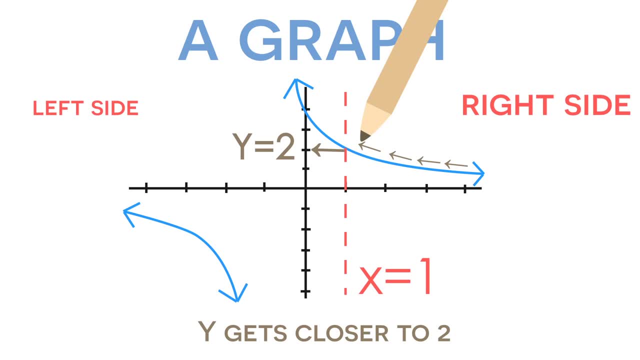 So now let's do the same thing from the left side of x equals 1.. If we put our pencil on the graph and we draw arrows from left to right towards the line x equals 1, notice, as we approach 1, as we get closer and closer to the line x equals. 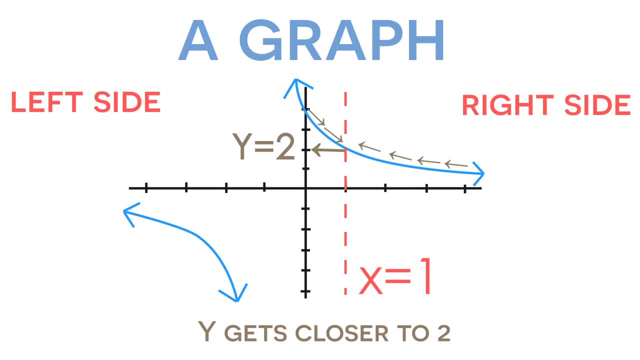 1, the y value gets infinitely closer to 2.. So the y value is the same as x approaches 1 from the right and from the left. So this is really interesting. Thanks for watching important and you should probably write this down if you haven't done so already. 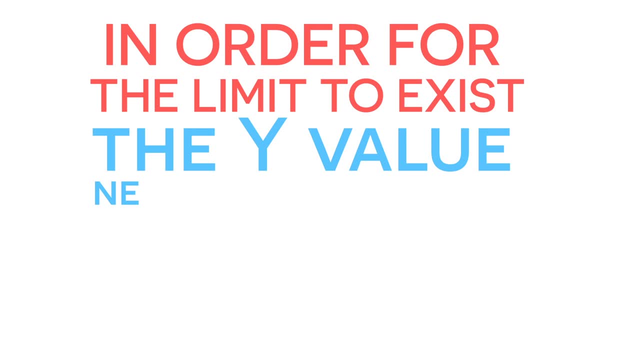 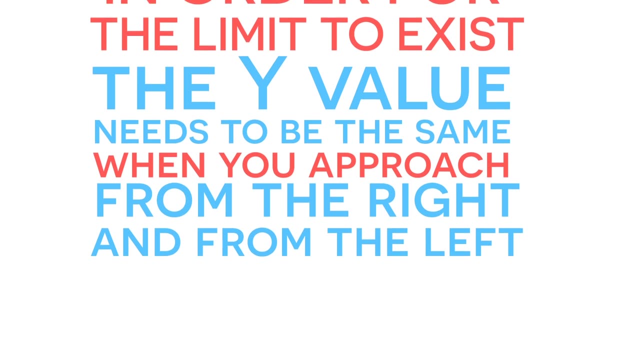 In order for the limit to exist, the y-value needs to be the same when you approach from the right and from the left. So, for this particular example, our y-value is the same when we approach from the right and when we approached from the left. 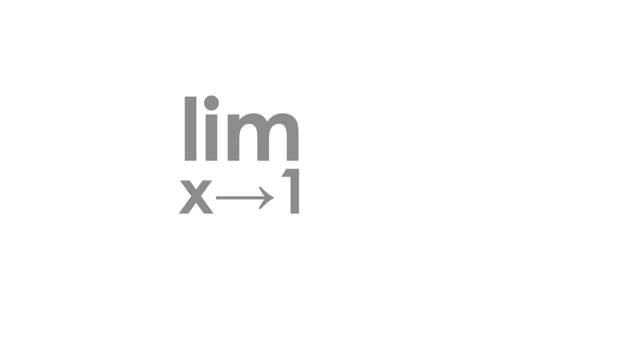 Because it was the same. we could say: the limit as x approaches, 1 is equal to 2.. Now the reason why I solved this for you using a graph is because I wanted to visually explain to you what a limit really is. But we could have solved this problem very easily algebraically. 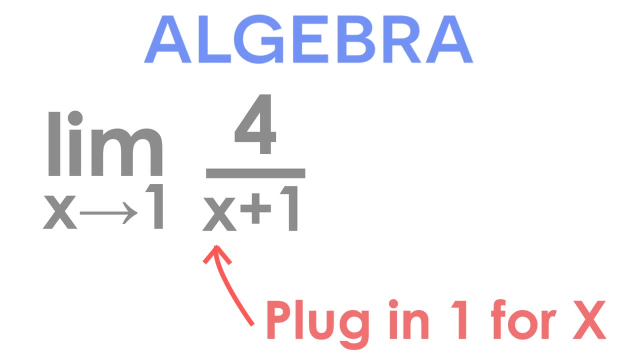 Since x is approaching 1, we could plug in 1 for x and we get 4 over 1 plus 1 is equal to 2.. So once again, the limit as x approaches 1 is equal to 2.. But most of the time the limit as x approaches 1 is equal to 2..